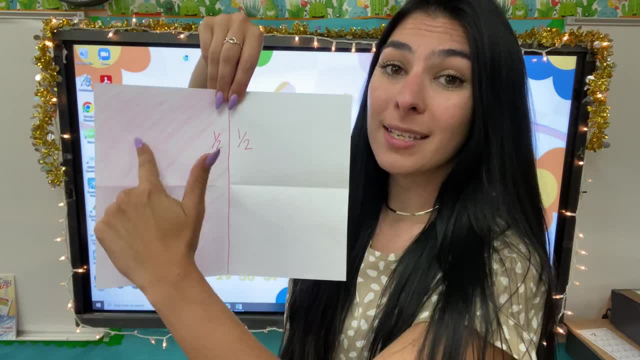 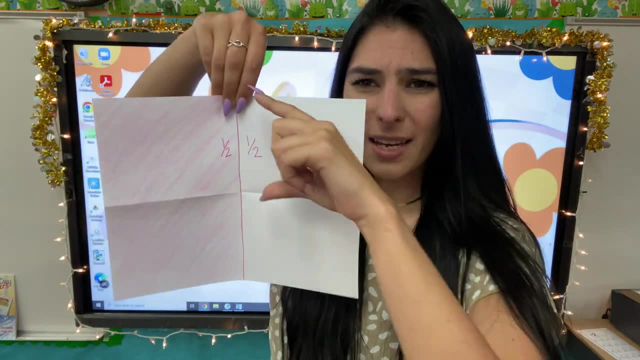 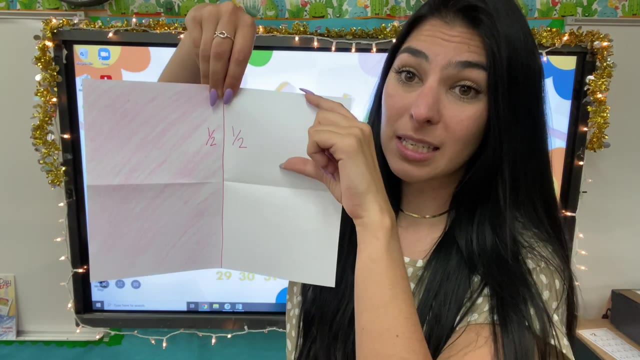 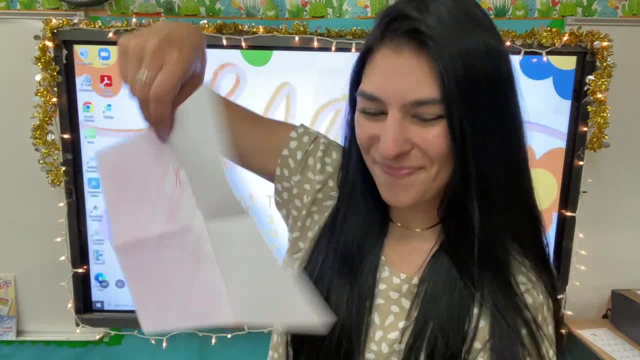 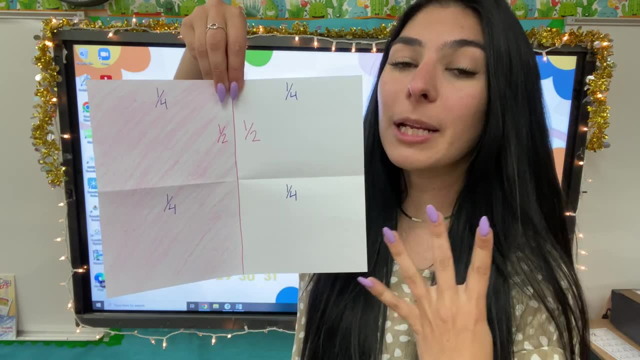 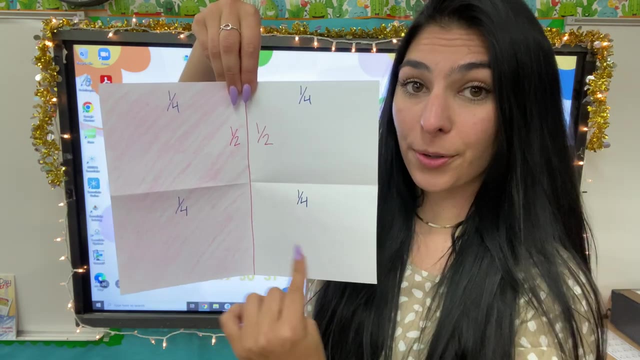 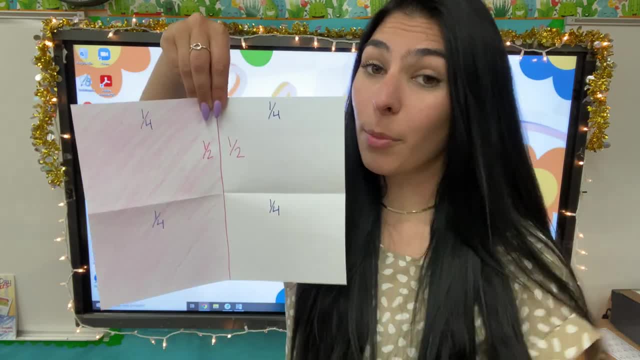 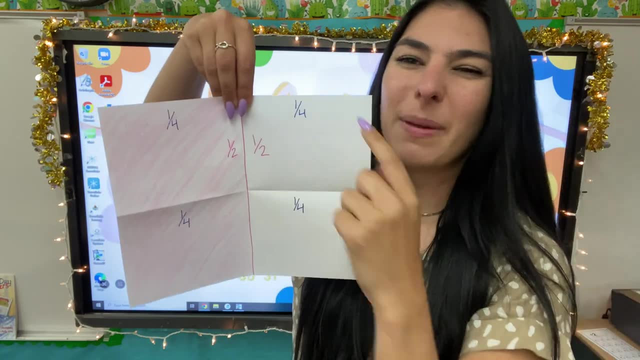 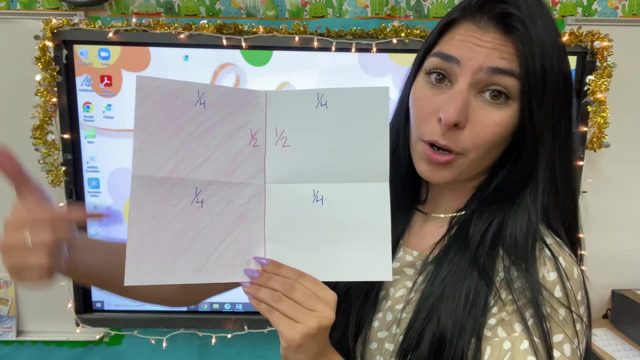 one piece. So the numerator in all of them is one. Remember: the numerator is on top, denominator is on the bottom. Denominator is how many pieces there are. The numerator is how many pieces we are talking about exactly. So, speaking of pieces, how many pieces? do I need to still have half my paper colored, Do I? 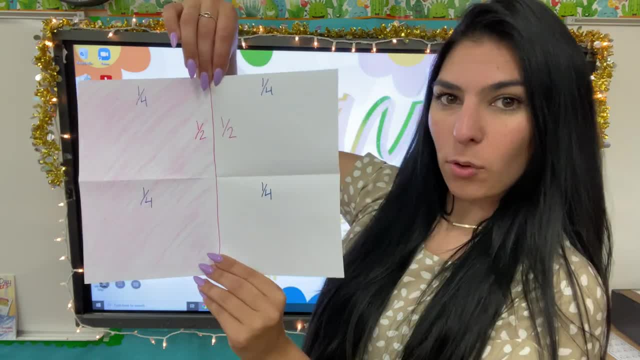 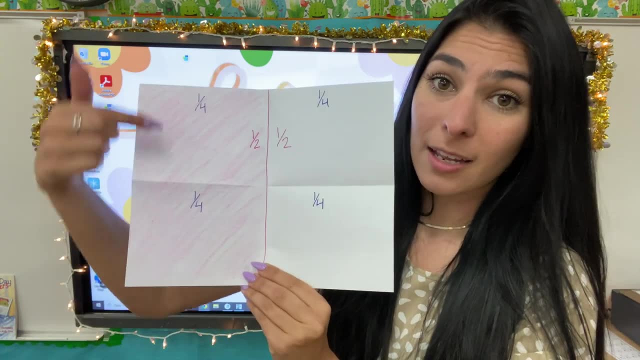 need just one fourth, two fourths, three fourths, four, fourths, two fourths. So look where we colored half of our paper, this pink side. how many fourths are colored in that half piece of paper? I have one. 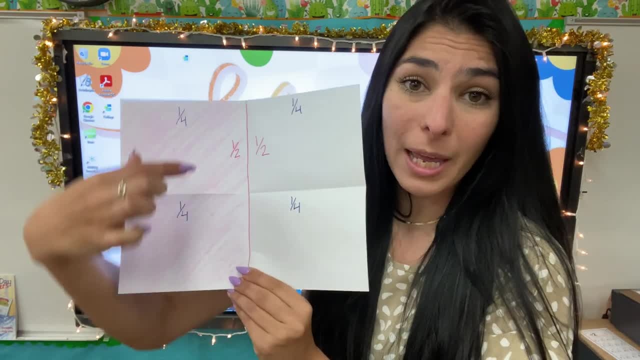 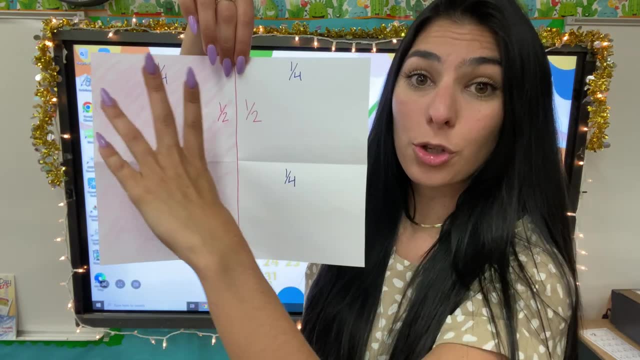 two pieces are colored, So that's one fourth, two fourths, three fourths, three, fourths, three, fourths colors. So in order to still have half our paper colored, our equivalent to one half is two-fourths, because one piece, two piece, Two-fourths is the same as one half. Now we're not done, Let's keep. 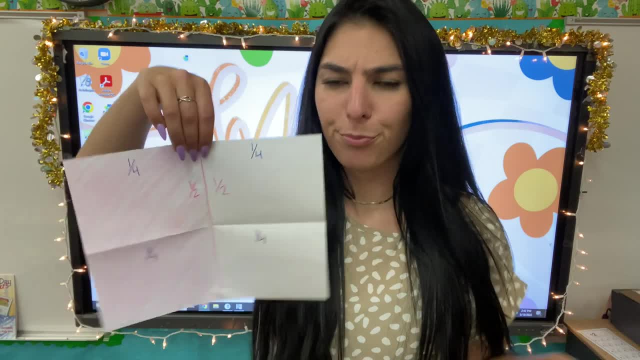 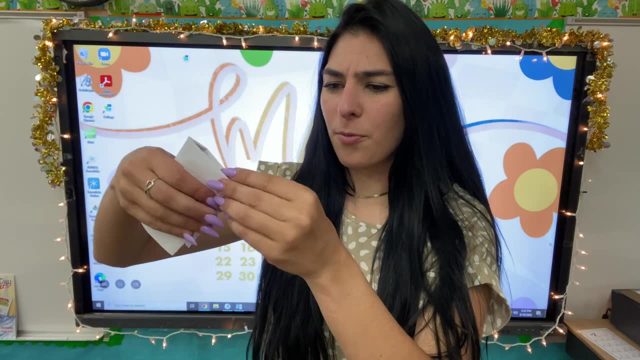 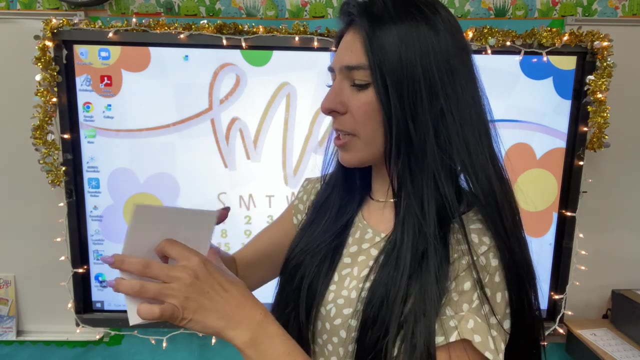 on going. We're going to fold it three times. this time You ready? Let's go One, two and one more. fold for three Now when we unfold it. So now that I've folded it a third time, I'm going to go ahead and 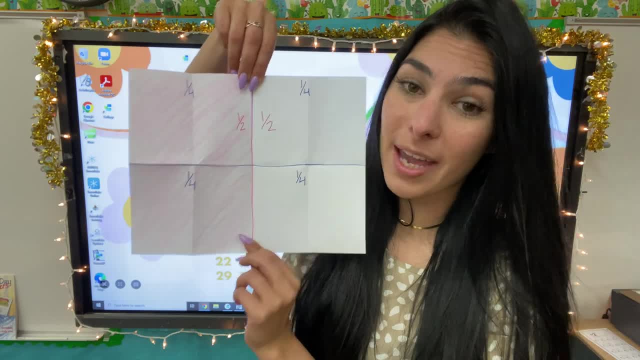 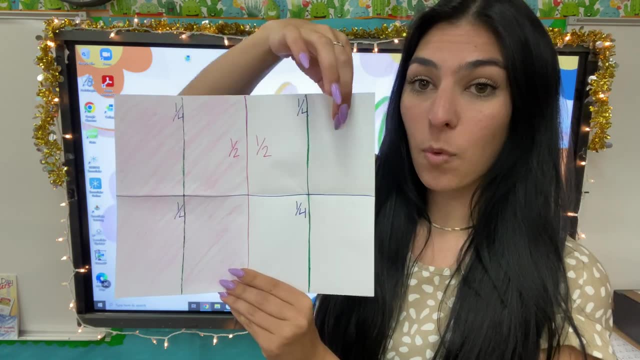 draw my lines so you can see it a little bit clearer and we can count how many pieces we have. Okay, so now I've drawn my more clear lines, Let's count how many pieces we have now that we've folded our paper. I have one, two, three, four, five, six, seven, eight, So that means our denominator.